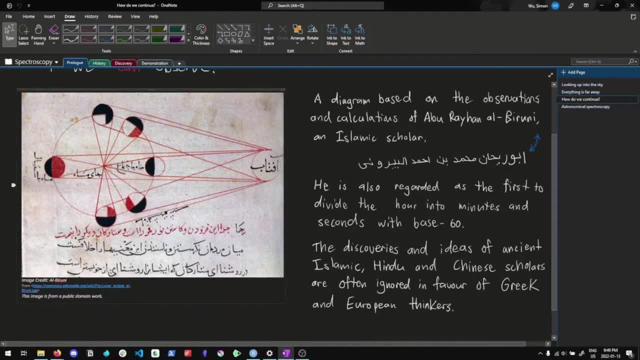 For example, I've got here a diagram of the phases of the moon which was drawn by an Islamic scholar named Abu Rehan al-Biruni. Al-Biruni was trying to understand the phases of the moon within the context of just what he could see from here on Earth And as equipment. 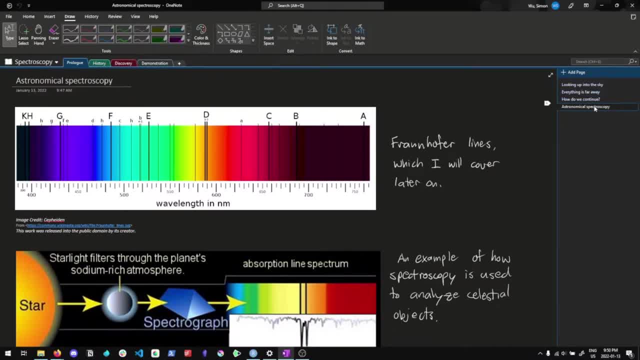 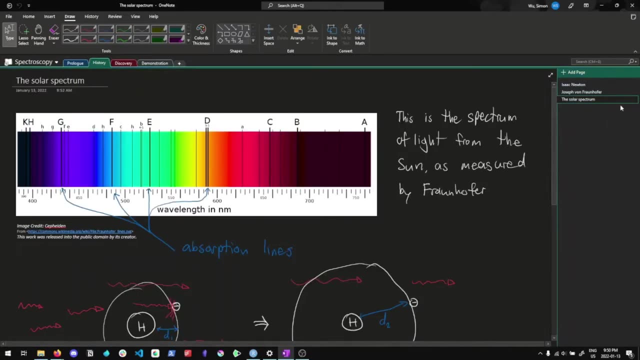 has gotten more advanced and sophisticated. the things that we can observe from here on Earth have gotten more sophisticated and advanced, And one of these things is light spectra, And from this has come the field of astronomical spectroscopy, which is what I'm going to be covering today: Spectroscopy as a field, really. 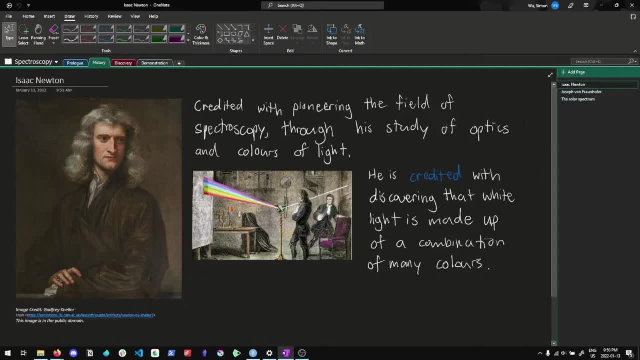 started with Isaac Newton. He is credited, of course, with discovering that white light, such as that emitted from the sun, is actually made up of different colors of light. He did this by separating it with a prism and then recombining it with a prism and doing all. 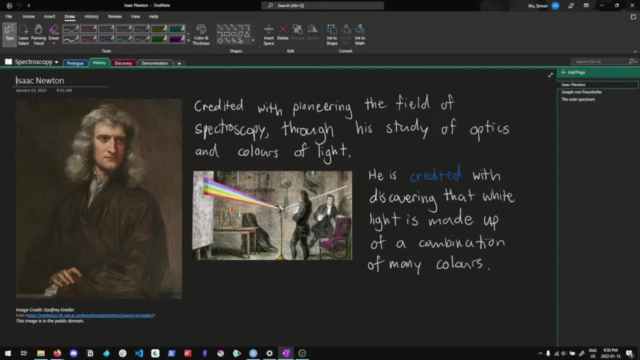 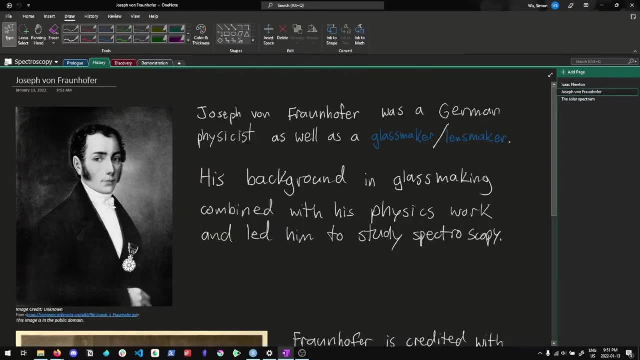 sorts of experiments with it. He observed this spectrum of colors coming from the prism. of course, that is actually visible spectrum of light. His findings on the spectrum of light spurred on a new interest in the study of the spectrum of light, especially specifically that coming from the sun. Joseph, 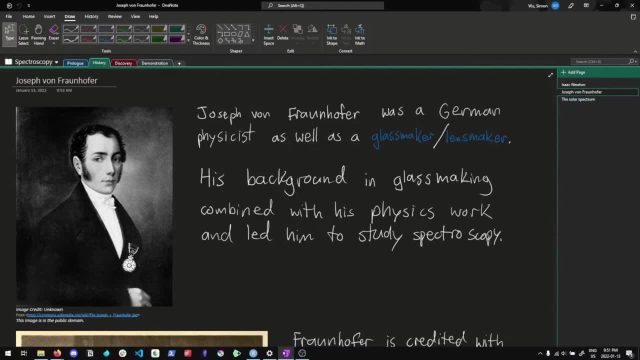 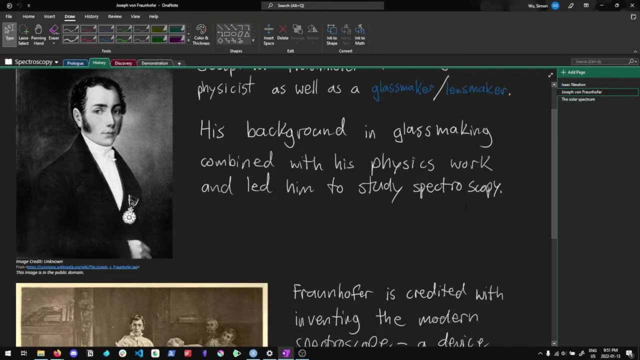 von Fraunhofer was someone who got really interested in this. He was actually trained as a glass maker, and so he had the skills to make very, very pure prisms for the study of optics and spectroscopy- essentially the first modern spectroscope which is a device used to view light spectrum. 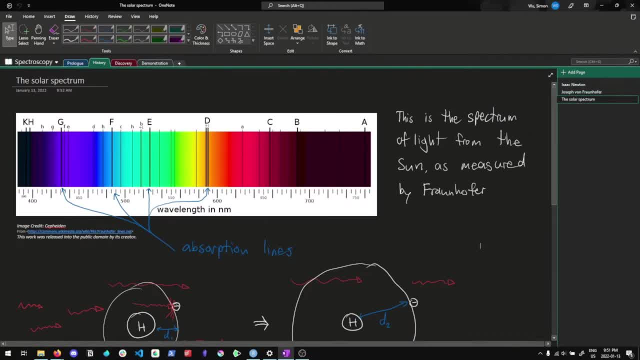 He used this to do a lot of things, and one of these was to observe the sun, and when he observed the sun, he found that the spectrum of light coming from it had a lot of these dark lines in it. He counted 574 of them in total and found that they were fixed on their position in 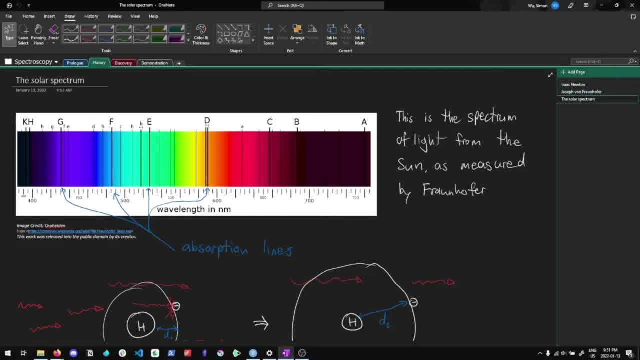 the spectrum from day to day. He also observed the spectra of stars in the night sky using telescopes with his spectroscope, and found that they also had these dark lines, but that they were slightly differently arranged. As it turns out, these dark lines he was observing were absorption lines. 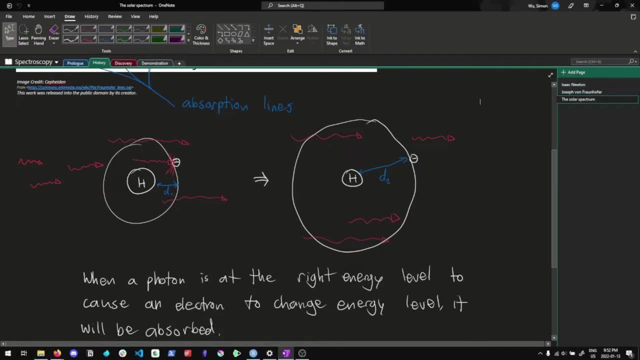 What these come from is the absorption of very specific wavelengths of light by atoms. For example, I've drawn this hydrogen atom here. As it turns out, when a particular photon of a particular wavelength of light strikes that atom, it has a very specific energy and if it's the right kind of energy it will. 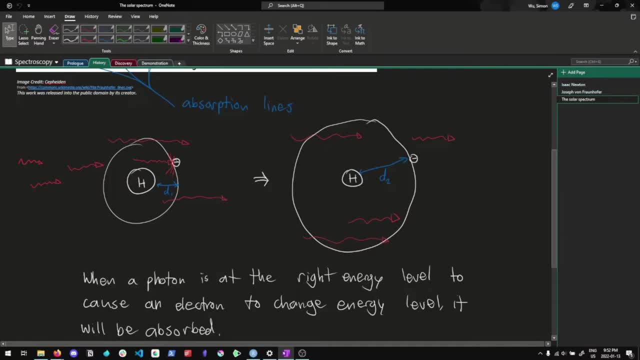 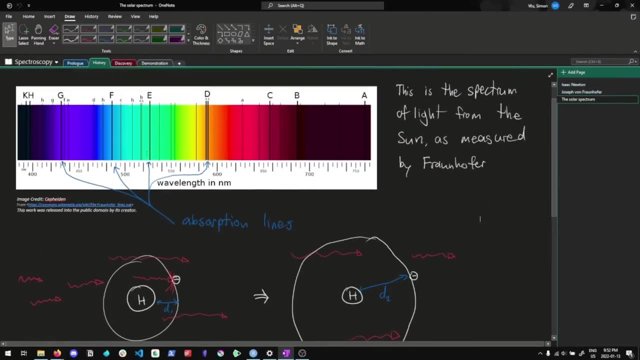 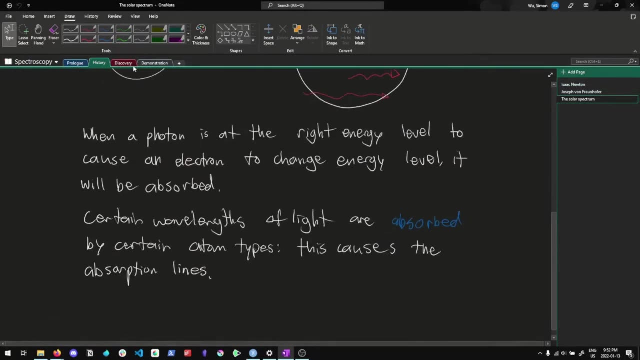 cause a very specific energy. It will cause an electron that is orbiting this atom to jump to a different orbital. This absorbs that photon into the atom and causes these absorption lines to occur, because all of those photons just aren't making it past. 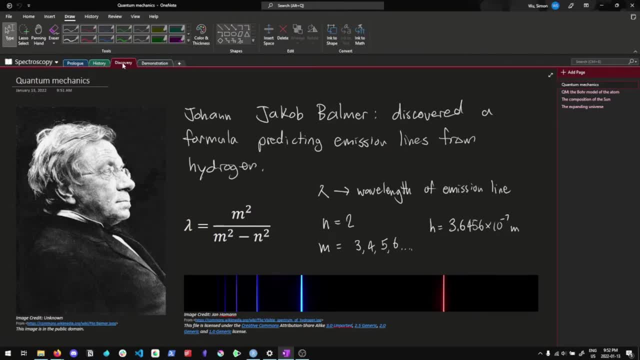 Stemming. from spectroscopy came a lot of different discoveries in the physics world, not just related to astronomy, but many of them, of course, related to astronomy. Johann Jacob Balmer, for example, discovered a formula for predicting the emission lines coming from hydrogen. 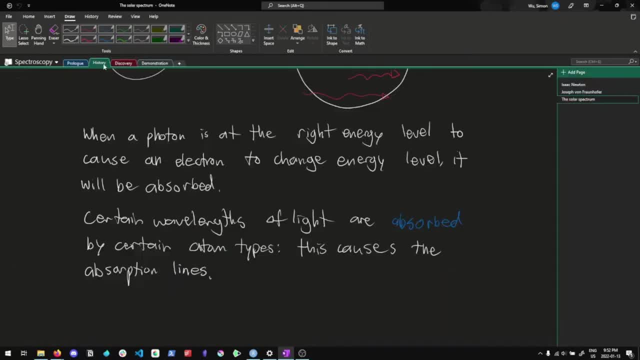 Hydrogen, which is what I mentioned here before, actually has emission lines, when you heat it up or otherwise energize it, which are actually the same, at the same wavelengths as these absorption lines. You see, once you energize it and it absorbs those particular wavelengths of light, it 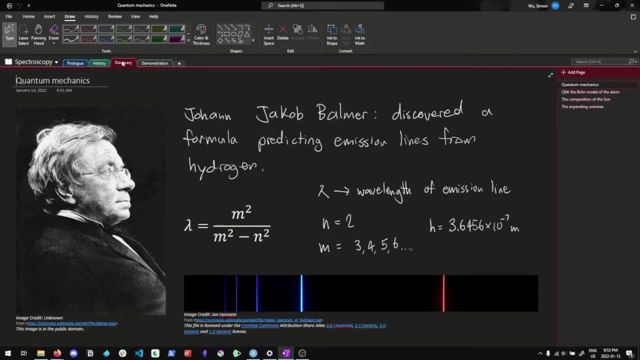 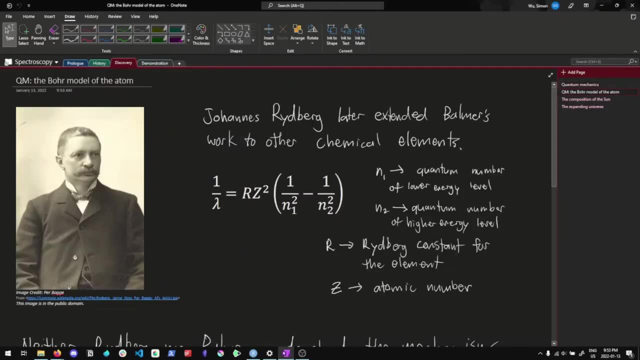 will actually re-emit them when those electrons go from those orbitals back to their lower orbitals. Later on, Rydberg: Johannes Rydberg created this formula for predicting the emission lines and created the Rydberg formula and extended these emission line predictions to other chemical. 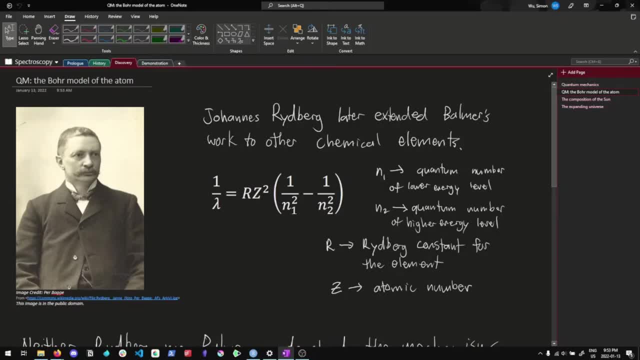 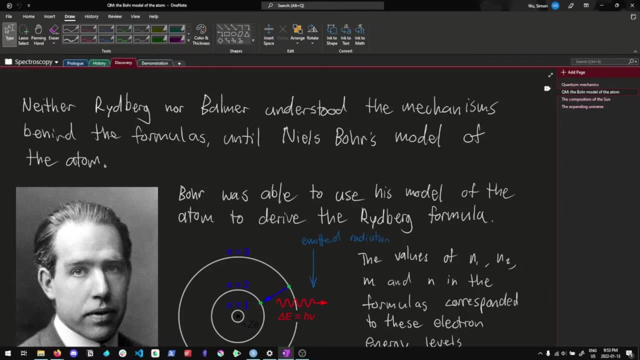 elements by taking into account things like the atomic atom. But neither Balmer nor Rydberg actually understood the mechanisms behind these formulas and no one really did until Niels Bohr and the model of the atom. You see, he was actually able to use his model of the atom to derive the Rydberg formula. 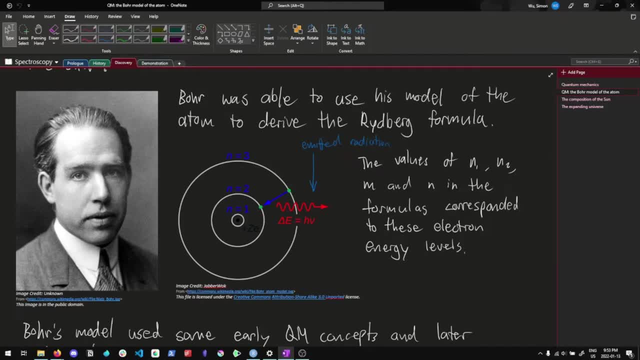 and love the constants within it, and he was able to describe the behaviors of these formulas very well. In the behavior of the atom, he was able to derive the Rydberg formula and love the constants within it. He used Rydberg to infer that there is a constant heat at a given point. 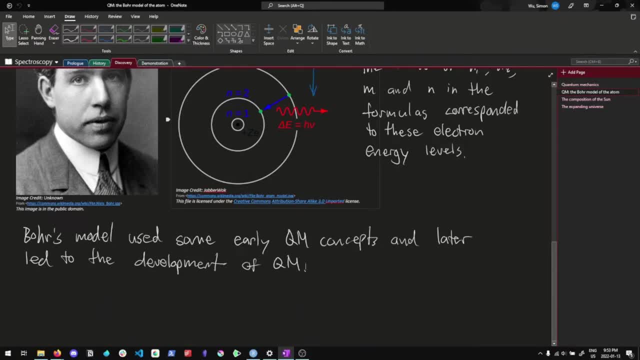 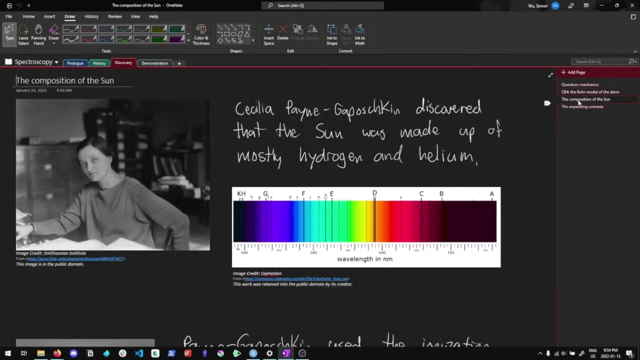 So instead of using the Rydberg formula only for inner force, he just began toЗ Fake-otic, because S and X are all the same pretty similar to that of Earth. But Cecilia Payne Kaposchkin actually did a lot of observations. 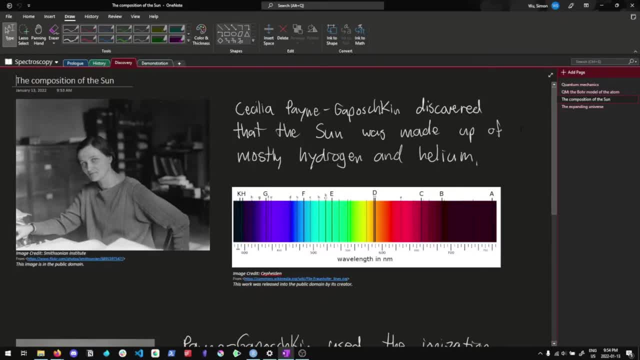 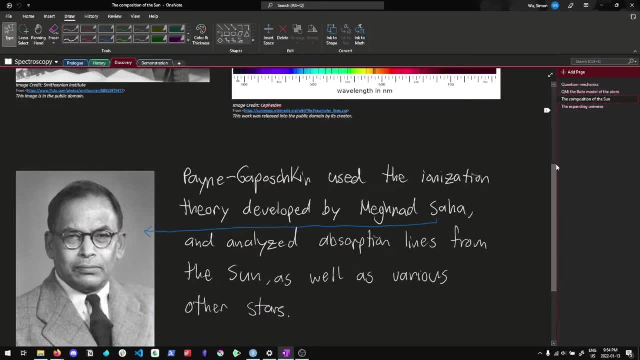 and research and found that this wasn't really true. In her doctoral thesis, she applied the ionization theories developed by Meghnad Saha, who was an Indian astrophysicist, and analyzed stellar absorption lines from the Sun and other stars using these theories. 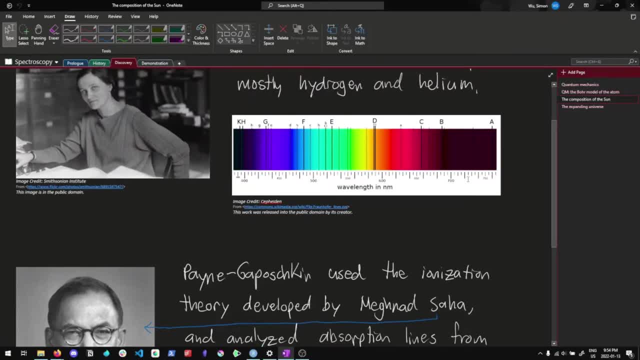 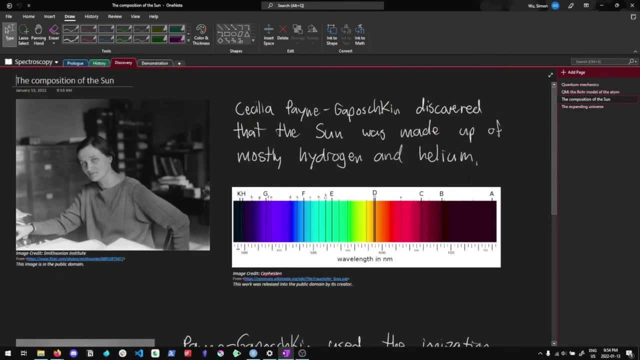 and found that stars such as the Sun were made up mostly of hydrogen and helium. However, Henry Norris Russell, who was reading her dissertation, actually dissuaded her from concluding this because it went against the scientific consensus. About four years later, though, he realized that she was actually right about the Sun being made up mostly of 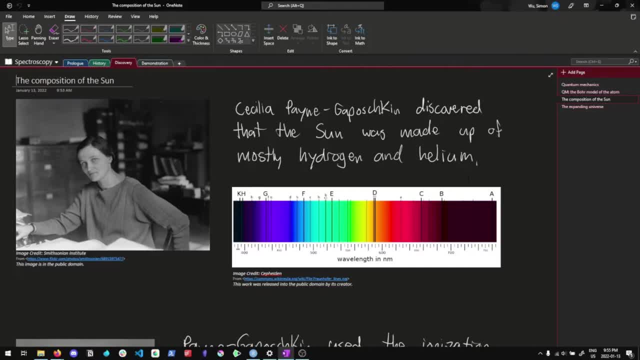 hydrogen and helium and actually published something about this, crediting her specifically with discovering this. However, of course, because Cecilia was a woman, Russell actually ended up sometimes getting credited for this discovery instead of her History blows, I guess. 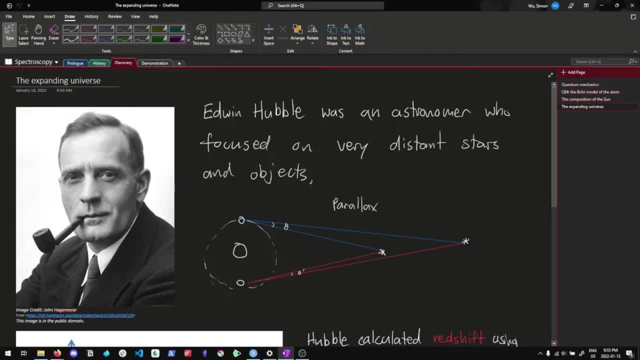 The final thing I'll be talking about today is the discovery of the Sun. The Sun is actually the expansion of the universe. Edwin Hubble was an astronomer who focused on very distant objects and stars in the sky. A lot of his work involved observing what he thought were. 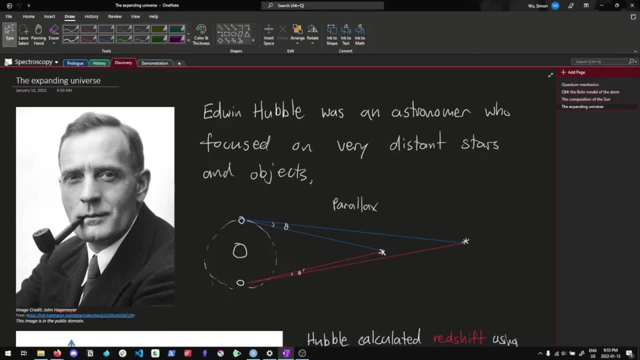 clouds of gas or dust in the sky, but what they actually were were galaxies beyond the Milky Way. As part of his work, he often observed the parallax of objects in the sky. Parallax is essentially the shift in the relative positions of stars in the sky as the Earth moves around. 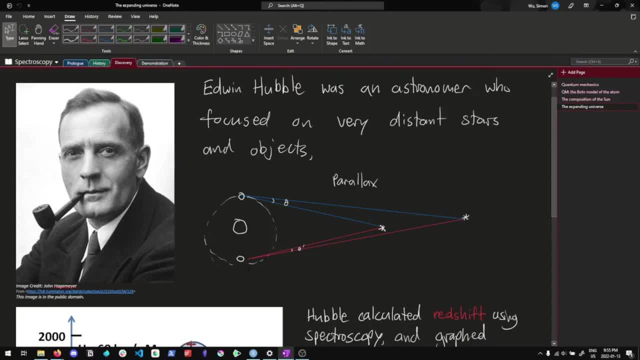 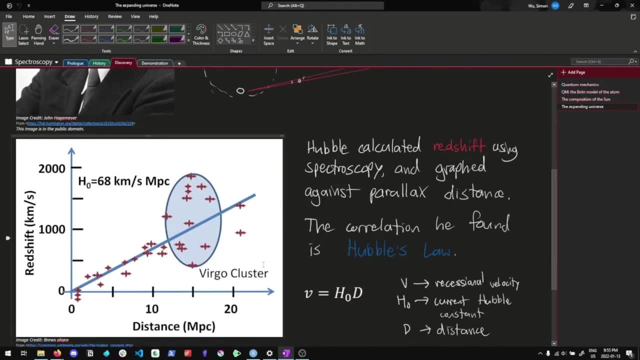 the Sun. Hubble also calculated the redshift of stars and other galaxies in the sky using spectroscopy. Basically, he looked at the absorption lines of these stars and found that they were shifted from the absorption lines that should have been there from various known elements and 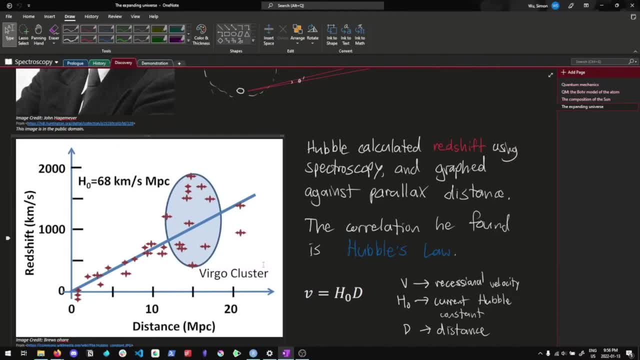 used this to determine the redshift, which was how much these wavelengths were shifted. You see, in this study, Hubble also found that these stars and galaxies were in fact, When things are moving away from us or towards us and they're emitting light, there's actually a Doppler shift, the experience that we can measure when we use something like a spectroscope. 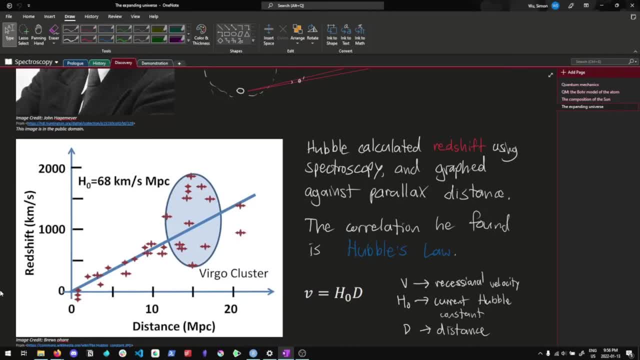 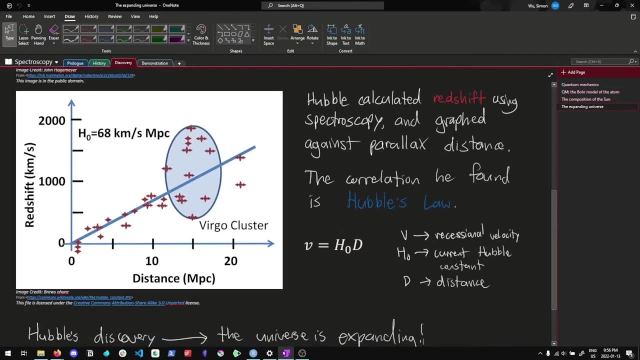 It's very similar to the Doppler shift you hear, for example, when there's a siren moving past you. And when he grabbed the redshift velocity that he calculated from this and the distance from Earth that he calculated with the parallax, he found this nearly linear relationship that he codified in the Hubble's Law. 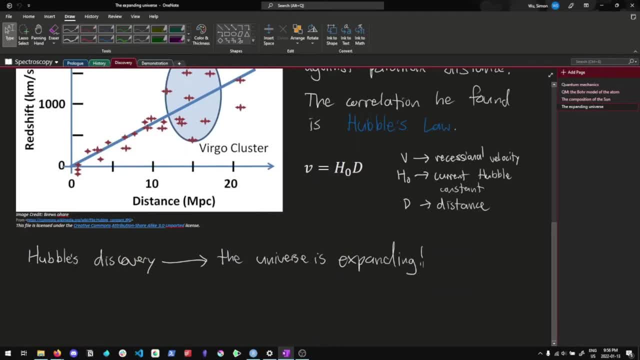 These findings, along with a lot of findings from other scientists at the time, led to the conclusion that the universe was actually expanding. In fact, we now know that the redshift of light from very distant galaxies isn't necessarily the same as the redshift of light from very distant galaxies. 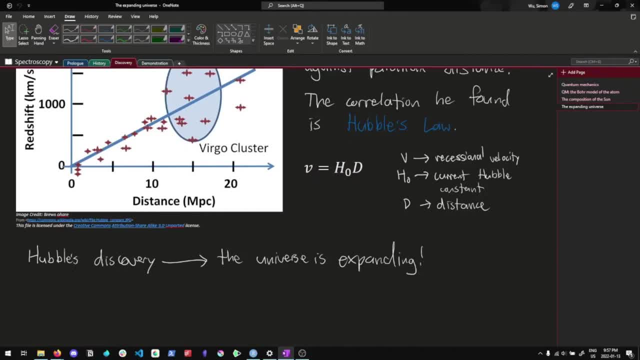 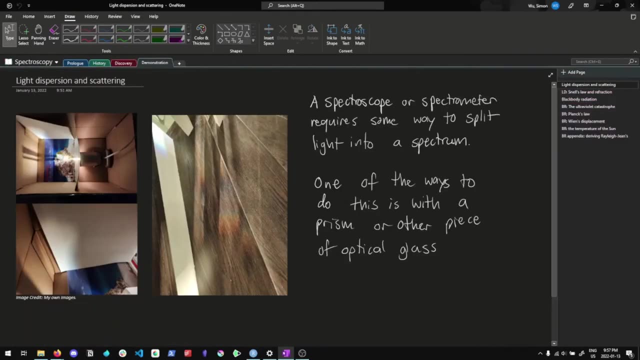 It's not necessarily from the fact that they're speeding away from us, but from how the light that is coming from them is actually literally getting stretched out because of the expansion of space and the universe. Now I'll be talking about some demonstrations and applications of the physics of spectroscopy. 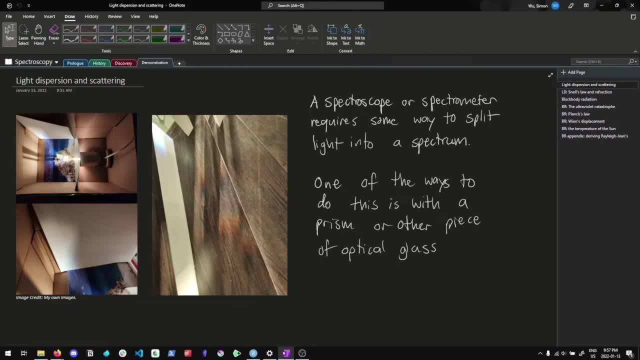 So spectroscopy often involves splitting light using prisms and other optical glass, For example. here I've got a picture of a prism and a spectrum that I managed to split from it, And this is just a picture of some stairs in my house that had some light cast on them from the sun through the window. 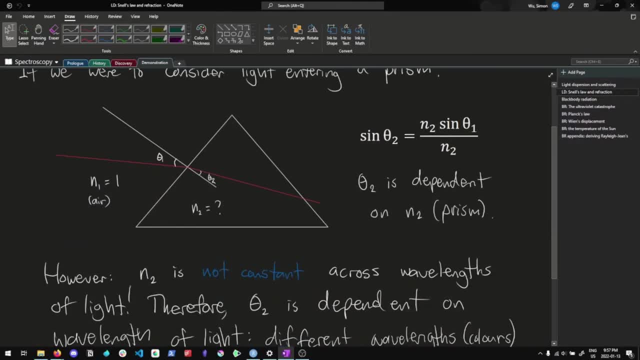 The reason that this occurs is because the index of refraction of light isn't actually completely constant for different wavelengths of light. It's actually dependent on the wavelength of light. For example, I have this Snell's Law calculation for light moving and refracting through this prism. 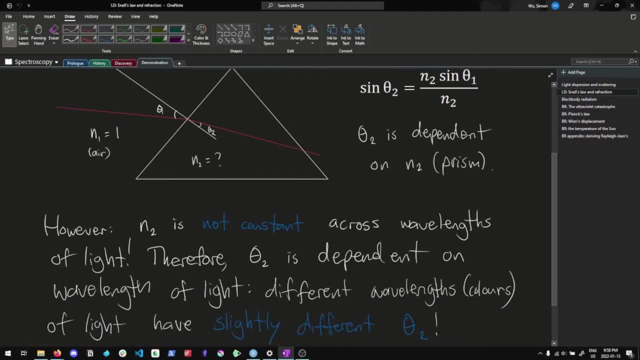 However, this n2 value isn't actually constant for all wavelengths of light. It's actually dependent on wavelengths of light and the color of the light because of that, And what happens is different colors of light will refract differently because of this. That's why Newton was able to split light through these prisms into different colors. 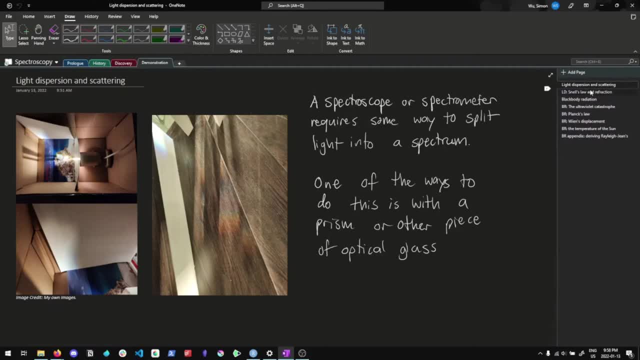 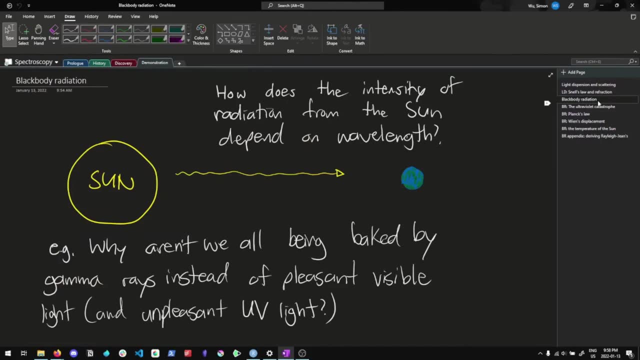 And why the light on my stairs and the light that I sent through these prisms split into a rainbow. Blackbody radiation is another concept very important to spectroscopy and physics in general. It relates the intensity of radiation to its weight. For example, there's a reason that the sun is mostly sending visible light, an ultraviolet light, at us, rather than gamma radiation killing us all. 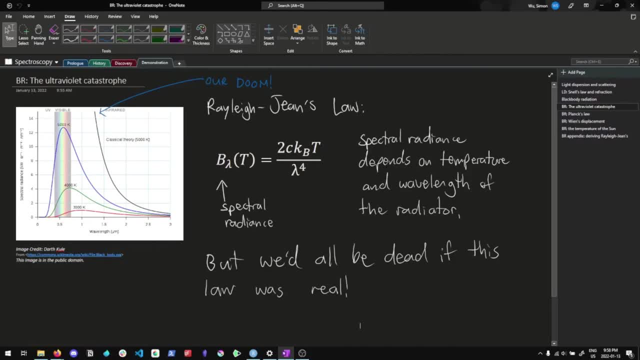 However, for the longest time we didn't really understand how this worked. We had the Rayleigh-Jeans law, which predicted that short wavelengths around the ultraviolet range, the irradiance of this light coming from a blackbody radiator would go to infinity. 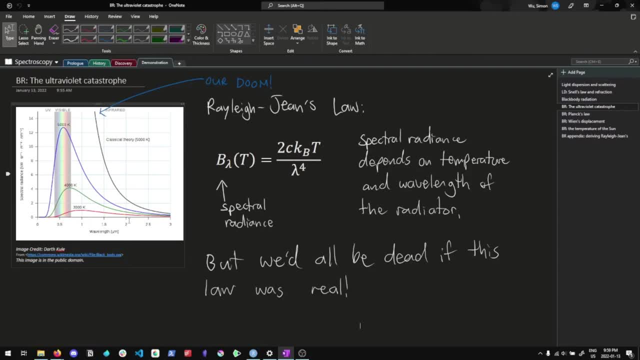 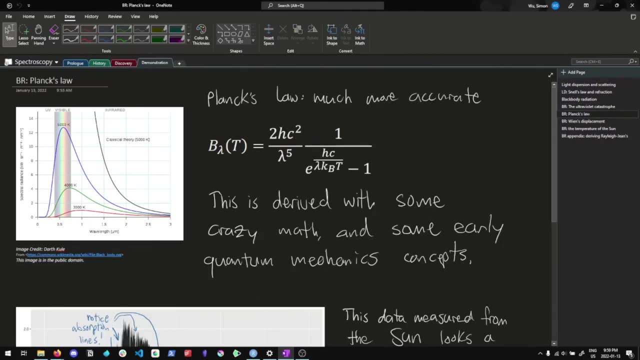 Obviously, this isn't happening because we'd be cooked and we'd be dead of cancer a hundred times over if this was true And eventually someone found a better law: Planck. Max Planck specifically- derived, using some crazy math and some thought experiments, essentially this new law that described our observations much more closely. 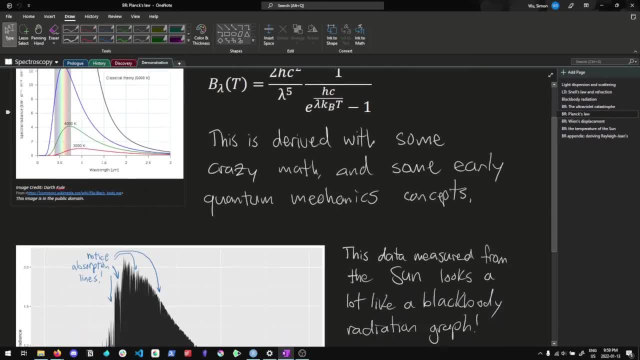 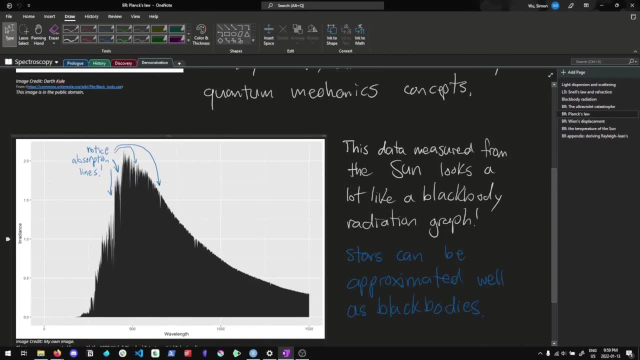 It creates these nice little graphs with peaks And, as it turns out, it also described what we know about stars pretty well. In this case, this is some data I have from the sun. I believe it's the 1985 Verily survey of the sun and its spectrum. 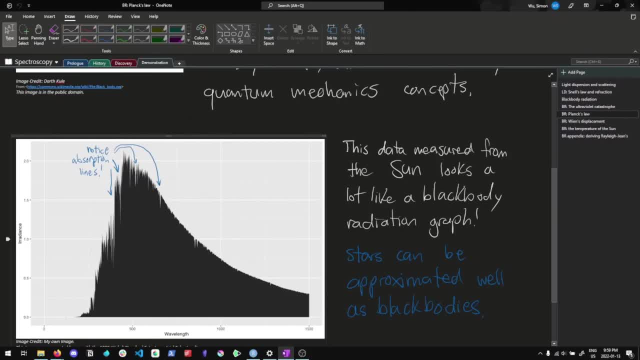 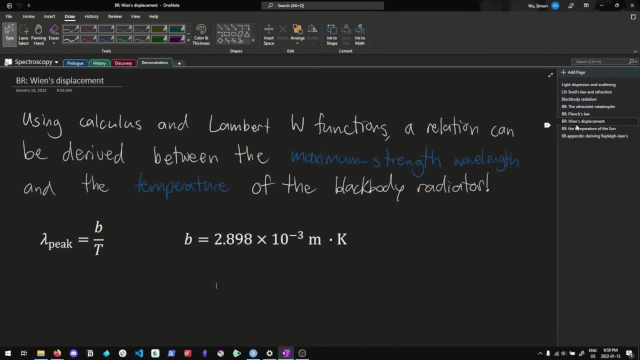 And we can see that there are some absorption lines in it, but that it matches the shape of these graphs generated by Planck's law pretty closely and very nicely. So how do we actually use Planck's law to determine properties of stars and other objects? 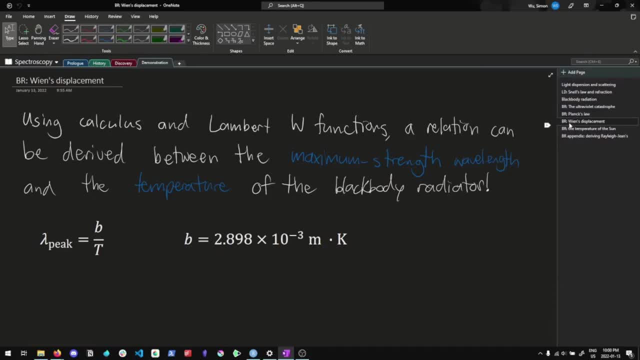 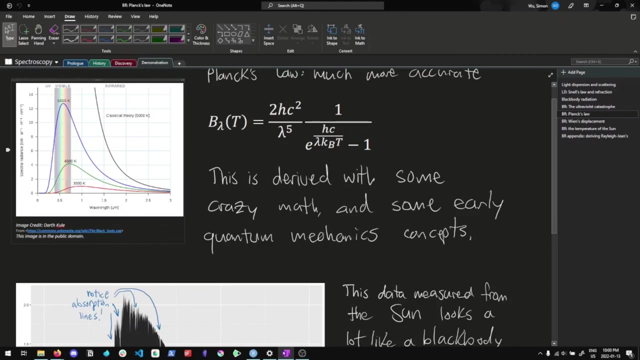 Well, we can use the Viennes this point. If you do a lot of terrible calculus and use some Lambert W functions, you can actually relate the maximum radiance wavelength, which is the wavelength at which the maximum radiance occurs, such as here: it's around 0.6 micrometers. 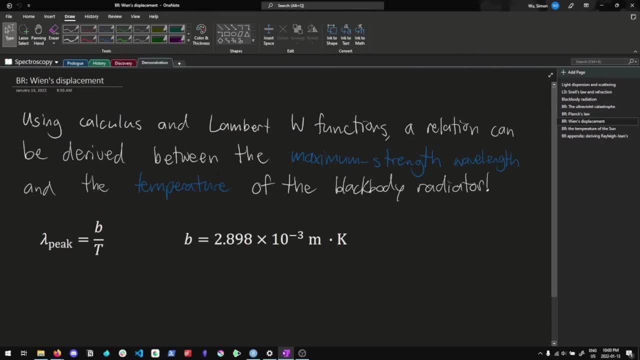 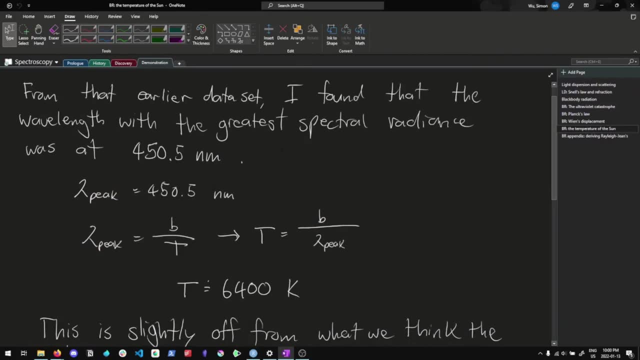 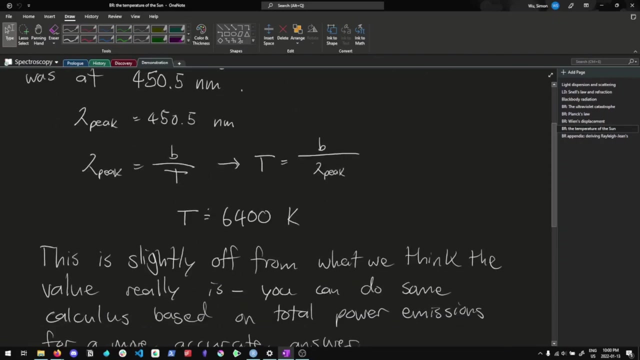 to the temperature of the blackbody radiator emitting that radiation. using this constant And if we do that for the sun, I pulled out the max radiance wavelength Using a spreadsheet program from that data and calculated this temperature. we can get some rough properties of the sun and other stars.